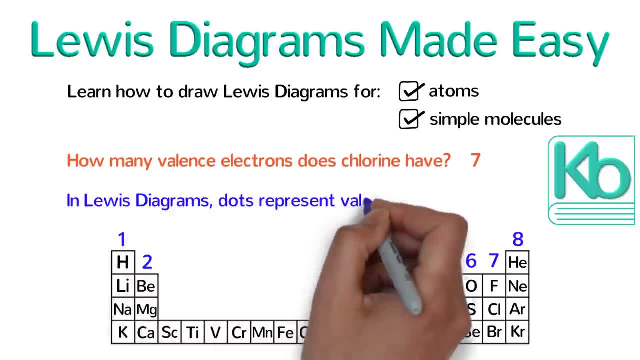 has is critical, and in Lewis diagrams we use dots to represent valence electrons. So the Lewis diagram of chlorine is the symbol Cl with 7 dots around it. When you draw the dots, don't just put them in. Instead, imagine a square around the element symbol. The dot should be neatly drawn on. 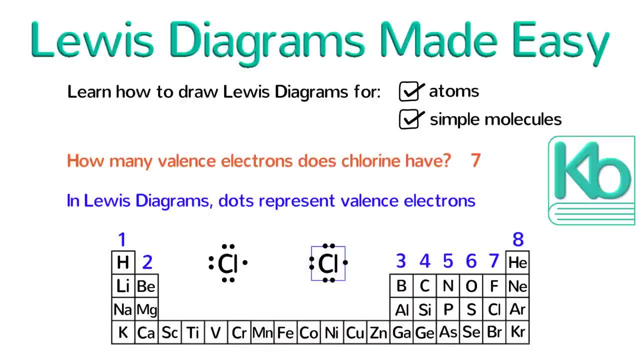 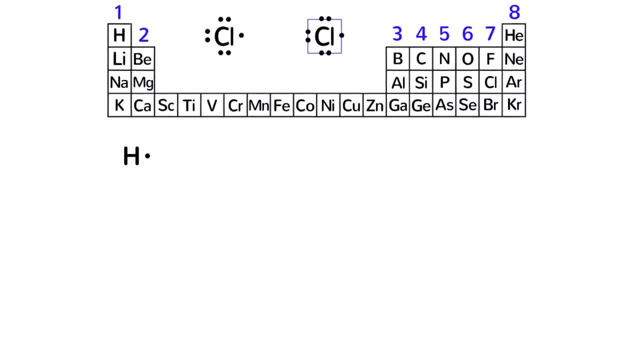 the 4 sides of the square, with no more than 2 dots on any side. Practice drawing Lewis diagrams of a few elements, just to make sure you've got it. This is the Lewis diagram of hydrogen, which has only 1 valence electron. This is carbon, which has 4 valence electrons. 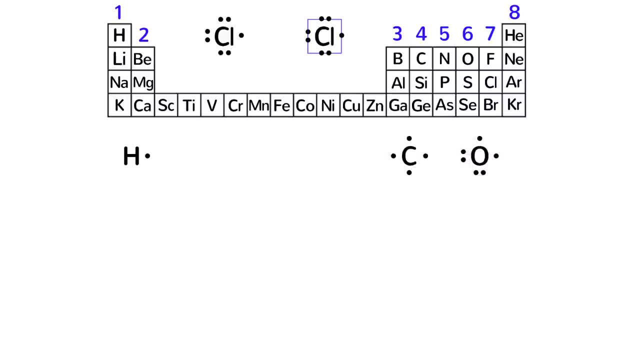 And this is oxygen, which has 6 valence electrons. Where you put the dots, it doesn't really matter, as long as you neatly draw them along the sides of an imaginary square and never draw them. Lewis diagrams are often used to represent covalent bonding in molecules. 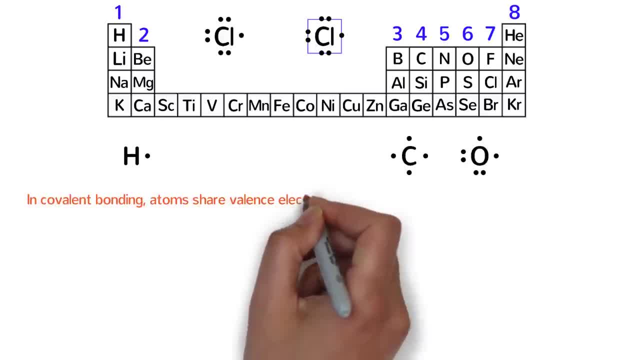 and ions. In covalent bonding atoms share valence electrons in order to get a full octet or duet. That is, every non-metal element wants 8 valence electrons, except for hydrogen, which only wants 2 valence electrons. The simplest molecule possible is that of hydrogen. 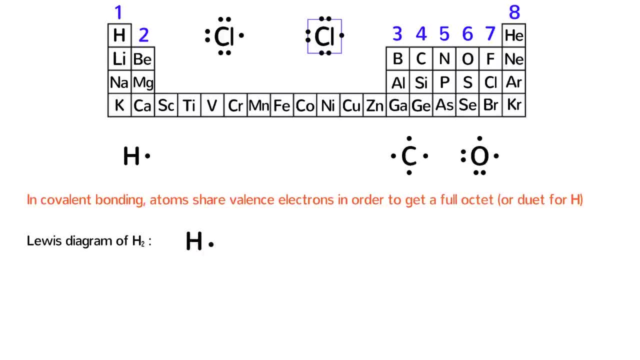 H2.. A hydrogen atom has one valence, electron, but it wants to have two. so in order to satisfy its desire for another electron, two hydrogen atoms will share their electrons with each other. And the crazy thing is that, in the wonderful world of atoms, the shared electrons 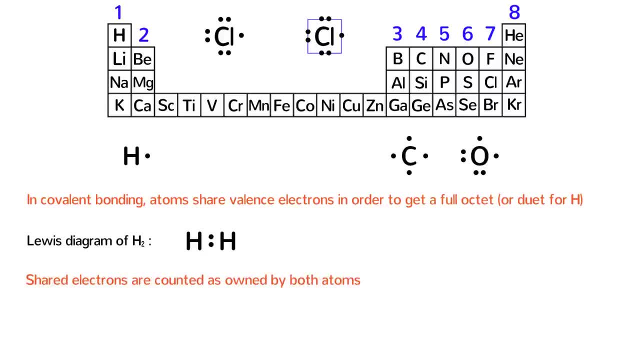 are counted as owned by both atoms. That means that both hydrogen atoms are happy because they both satisfy the octet rule. Now we normally draw hydrogen and other molecules like this with lines to represent shared electrons and dots only for non-bonding electrons. These 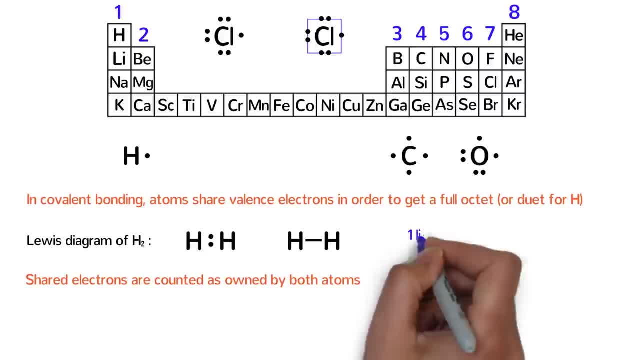 two diagrams of a hydrogen molecule are equivalent because one line, which is a single bond, represents two shared electrons. In the same way, two lines between atoms would be a double bond and would be the sharing of four electrons. An example of a molecule with a double bond. 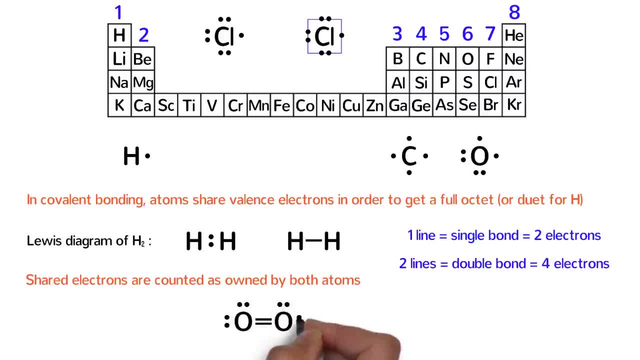 is oxygen, which looks like this. Notice that in this Lewis diagram both oxygen atoms have 8 valence electrons, 4 from the double bond and 4 from the lone pairs of electrons. By the way, two dots together are called a lone pair of electrons. Some molecules contain triple. 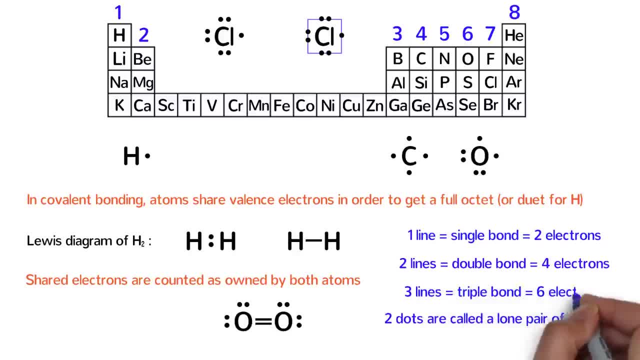 bonds, which we write using three lines that represent the sharing of 6 electrons. An example of a molecule with a triple bond is nitrogen, which looks like this: Once again, notice that both nitrogen atoms have 8 valence electrons, 6 from the triple bond and 2 from the lone. 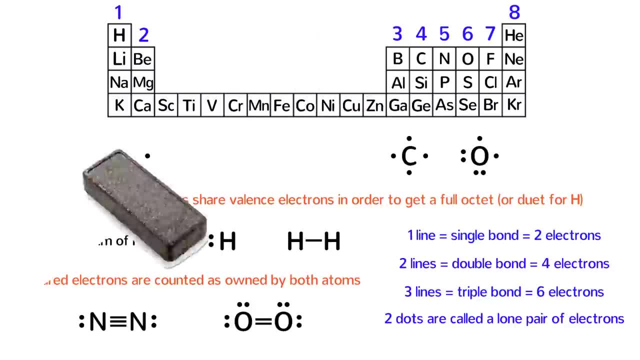 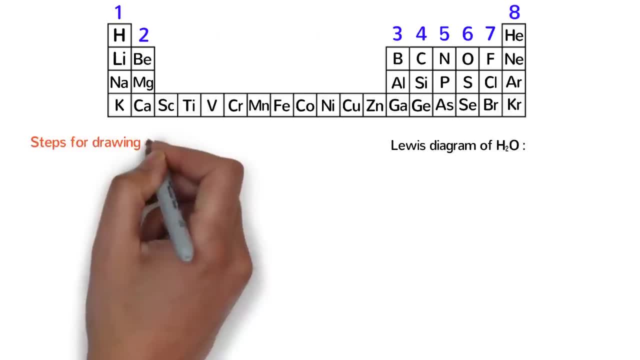 pair of electrons. Okay, how do you actually draw the Lewis diagram of a molecule? Let's start with water, H2O. There are five important steps that you need to follow when drawing the Lewis diagram of a molecule. First, count all of the valence electrons in the molecule For water, each. 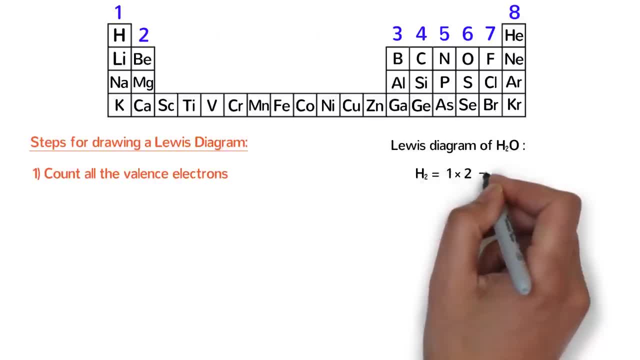 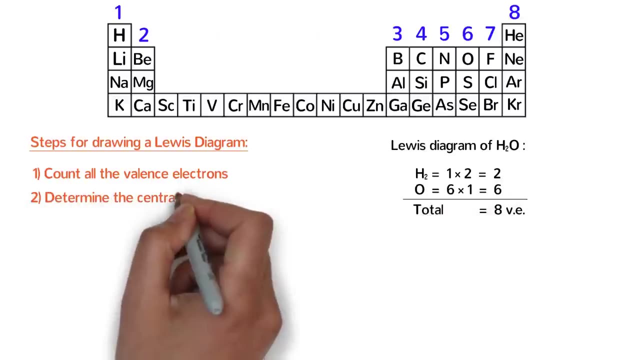 hydrogen has one electron and we multiply that by 2 because there are two hydrogens in the molecule, The oxygen has 6 valence electrons. Add those all up and we have a total of 8 valence electrons for the water molecule. Step 2, determine the central atom. 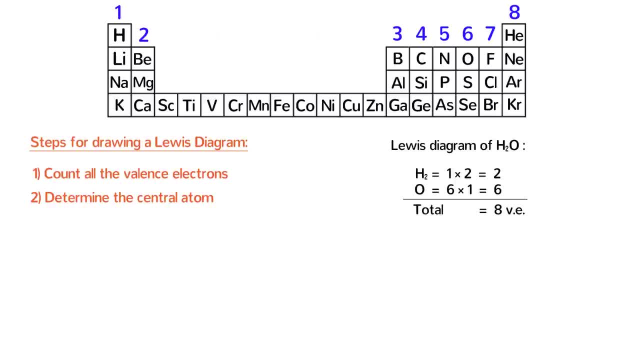 The central atom is the one that all the other atoms will be bonded to. It is usually the element that there is only one of. In the case of H2O, because there are two hydrogens and only one oxygen, we choose oxygen as the central atom and write it in the middle. 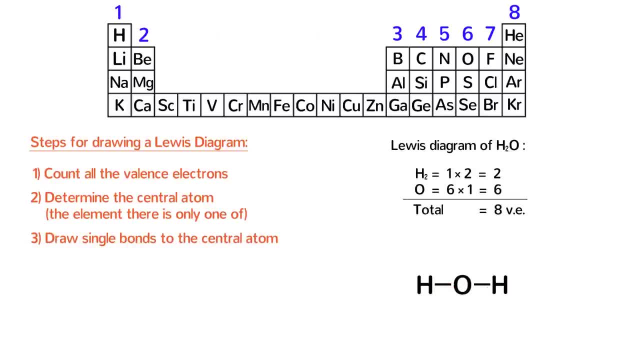 Step 3, draw single bonds to the central atom. Step 4, put all of the remaining valence electrons on atoms as lone pairs. For H2O we start with 8 valence electrons. We have used 4 valence. 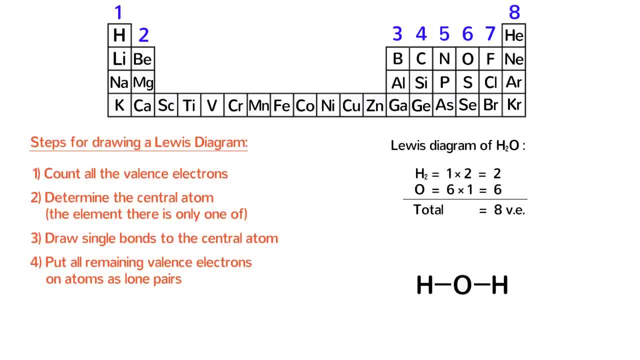 electrons for the two single bonds, so that leaves 4 more electrons left over. We put all 4 of these remaining electrons on oxygen instead of hydrogen, because hydrogen is already happy with 2 valence electrons. Remember, never give hydrogen more than 2 valence electrons. 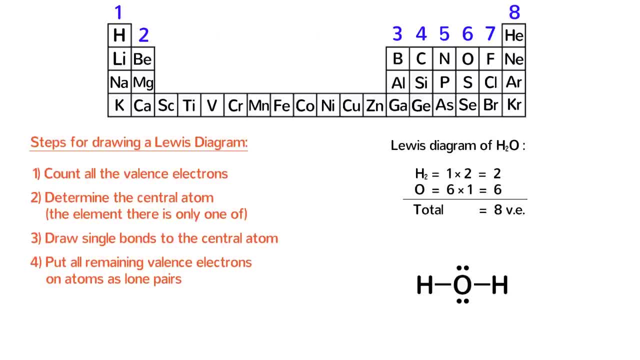 Everyone else wants 8 valence electrons, but hydrogen only wants 2.. Step 5, turn lone pairs into double or triple bonds to give every atom an extra valence electron. Step 6, add an octet or duet for hydrogen. Pause the video and see if all of the atoms in our H2O 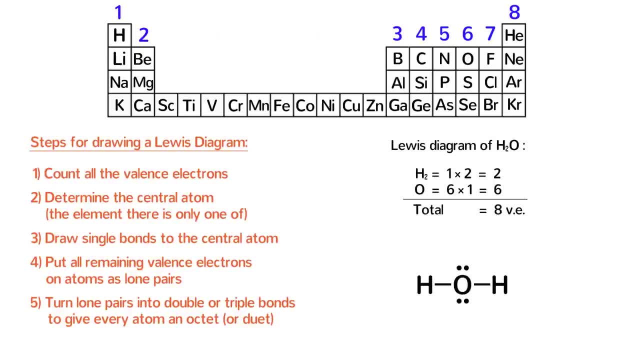 are happy, Because each hydrogen has 2 electrons and the oxygen has 8 electrons. everyone is happy and there is no need for double or triple bonds, which means that our Lewis diagram of water is now complete. Alright, let's try one more example, just to make sure that.